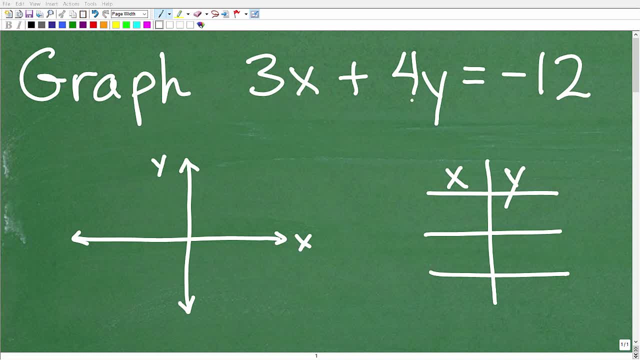 Okay, let's learn how to graph the line: 3x plus 4y equals negative 12.. So I'm going to go through that here in a second, And of course this is just one particular equation: 3x plus 4y equals negative 12.. 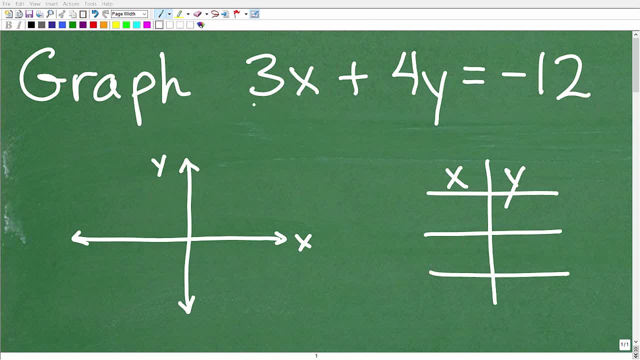 But obviously, what I'm going to try to teach you here is how to graph lines in this particular form, And we'll talk all about that in a second. First, let me go ahead and introduce myself. My name is John. I'm the founder of Tablet Class Math. 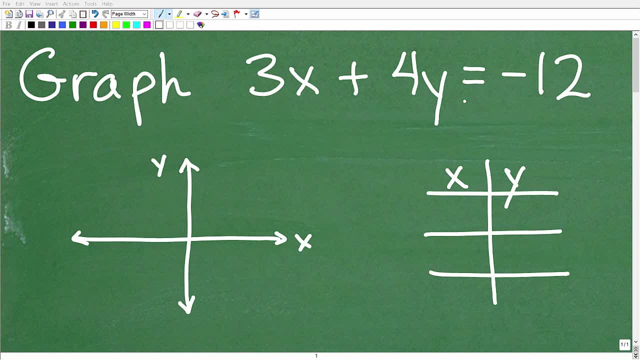 I'm also a middle and high school math teacher And over the last several years I've constructed many, many online math courses- rarely with super comprehensive instruction. So if you want to check out my math learning program, I'm going to leave a link to that in the description of this video. 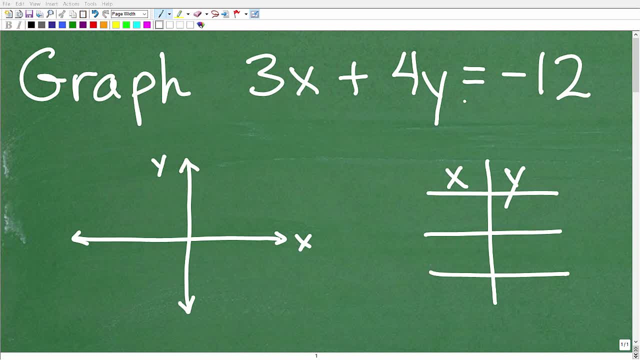 Again, you know, these things I do on YouTube, like this particular video, are quick tutorials just to try to get you out of a bind. You know, try to clear up any kind of confusion, But if you're really looking for a lot of math, 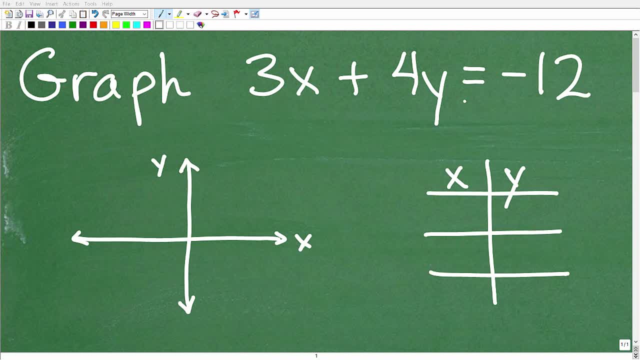 A lot of math help, a lot of examples, a lot of problems solved, etc. That type of thing. Then I'm going to encourage you to go ahead and check out my math learning program. Also, if you're new to my YouTube channel, I already have hundreds of videos on my YouTube channel that, if you like my teaching style, you can definitely check out on all kinds of variety of math topics. 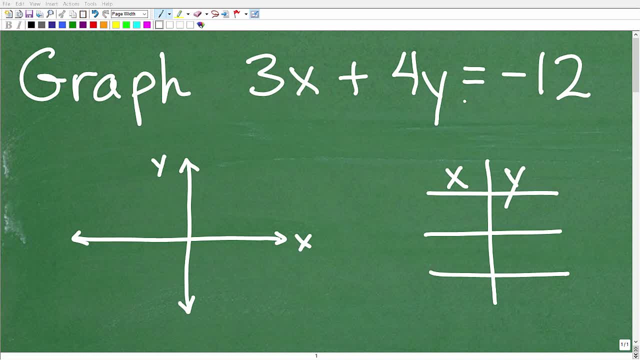 And if you like this video, please consider smashing that like button. So let's go ahead and get to it. Let's learn how to graph: 3x plus 4y equals negative 12.. All right, So here is our problem. 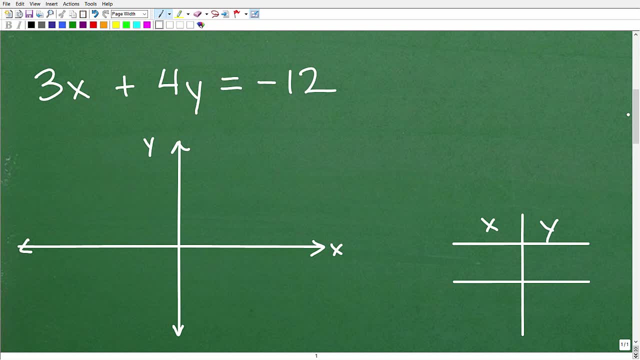 And this type of problem is really kind of fundamental to those of you out there that are kind of learning algebra, pre-algebra, algebra one, maybe college algebra, you know somewhere around this kind of level. But we learn these or we apply these skills in all math courses. 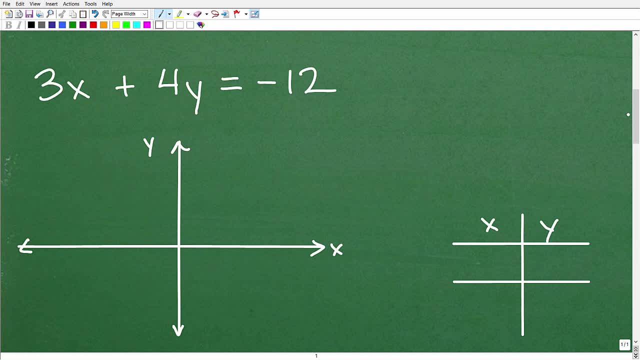 OK, so beyond, let's say you could be a calculus student. It doesn't make a difference. This is all you know. math builds upon itself, But typically You start learning this around. you know the middle school level. you know basic high school level mathematics. 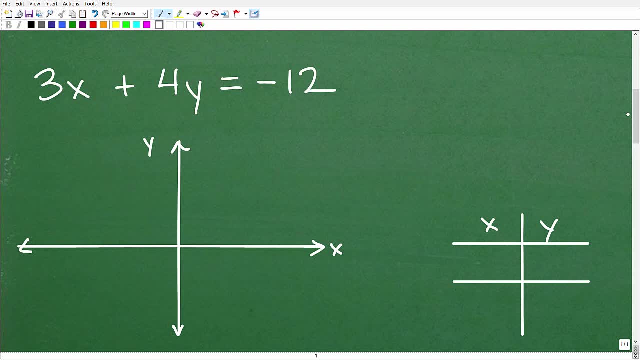 OK, now let's kind of consider what's going on here. So we have 3x plus 4y equals negative 12. So this, right here, is an equation. All right, It's an algebraic equation. We refer to equations like this in algebra as linear equations. 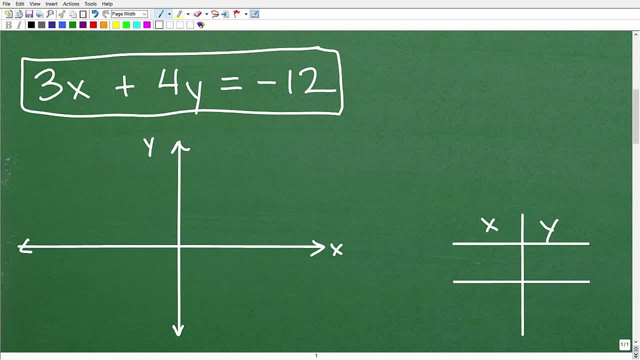 OK, meaning that this equation has a line associated with it, The graph. there's some sort of line, graphical representation of this equation. So what we're going to try to do is graph that line. All right, That's the whole idea here. 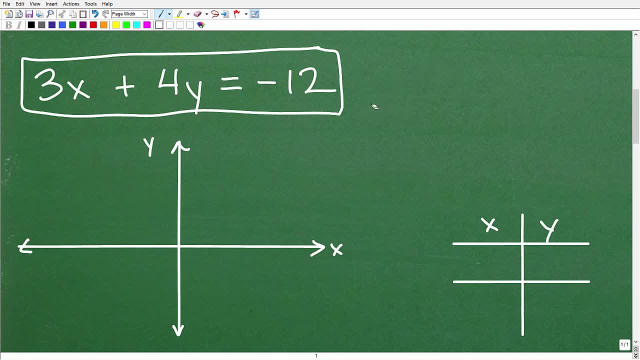 Now, one of the things that you can do when you're looking at this equation is: we have a couple options We're like: well, how can you graph a line in general, OK? well, we have a linear equation. It has both an X and a Y, like this: 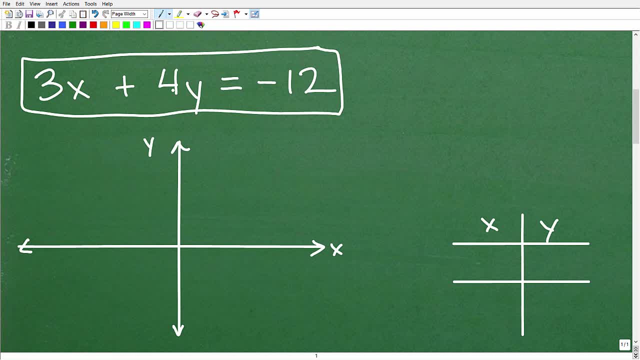 You pretty much kind of have three different kind of ways To kind of go about it, Right? So the first way is to always use some sort of table of values. This is kind of a basic table here. We're going to actually use that in this problem. 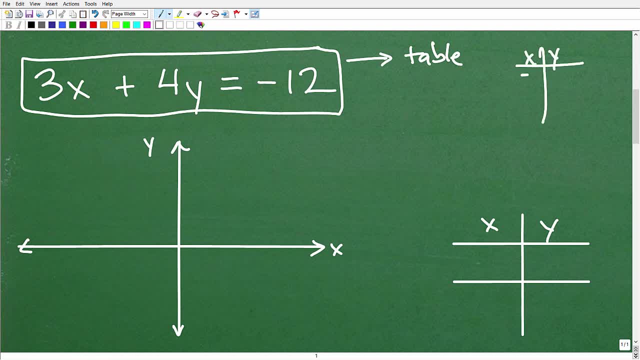 OK, but you can just make yourself an X- Y table, like so, and plug in a bunch of values for X, plug it all in and get a bunch of values for Y- These are going to be points that are on the line, OK- and then kind of connect the dots. 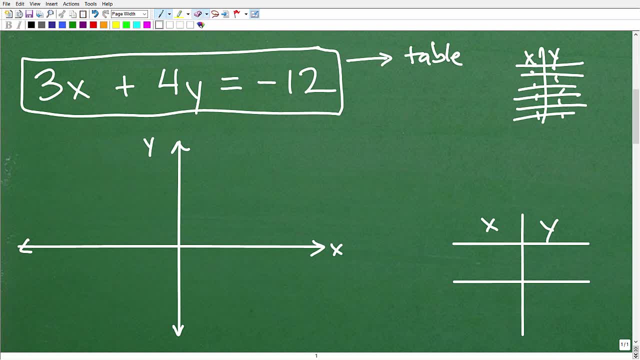 All right, Just draw a line through those respective points. But tables are, They're, they're good to know and you definitely need to know them. OK, but generally they're not the most direct path to graph a line. OK, so most linear equations, I would say probably. 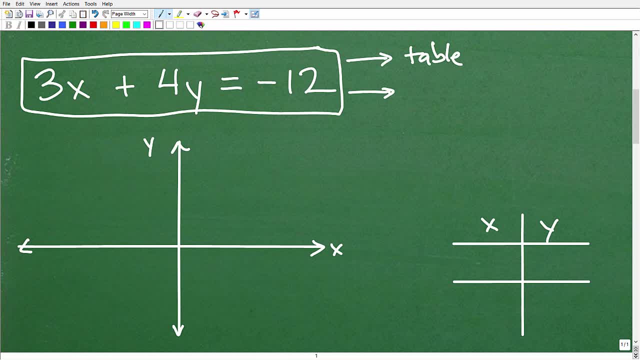 Well, yeah, I think I'm correct by saying this- that the majority of times when we're dealing with linear equations, we like to use the slope intercept form, the Y equals MX plus B form of a line. So if you're watching this video, I'm assuming that you're familiar with Y. 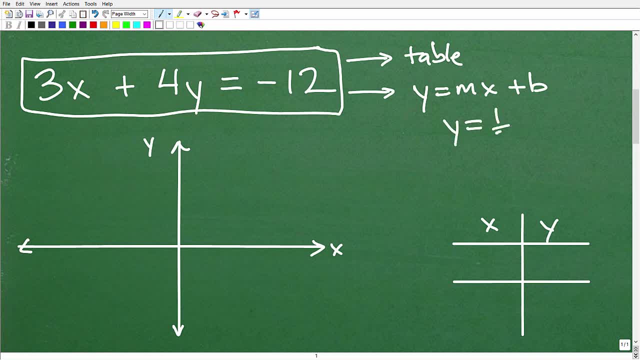 Y equals MX plus B. In other words, lines are like this: Y equals one half X plus five. You would know how to graph that line. OK, why would you know how to graph this line? Because you understand how the slope intercept formula works. 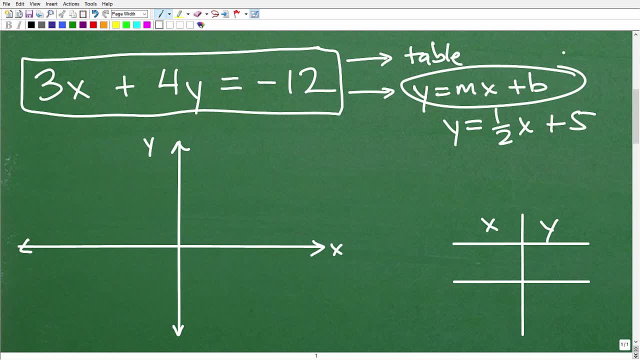 OK, so that's really important. You definitely need to understand the slope intercept formula and the basic mechanics of a table. All right, So that leaves us with this line. OK, you can also, if a line is in standard form, find the X. 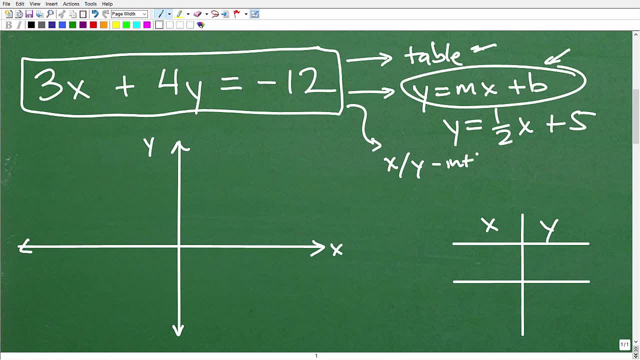 Y intercepts. OK. so this is kind of an abbreviated way of the table method. OK, it's kind of we're kind of doing something similar, but it's kind of its own technique, Right. So now we have these kind of three different paths that we can follow to graph this line. 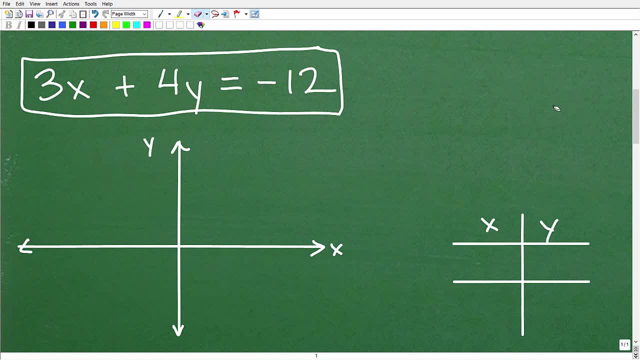 So we have three options here. So how do we know which is the right one? Well, really, you want to use the whatever technique, depending on what form the line is in, OK, In other words, what is the form Format of this line? 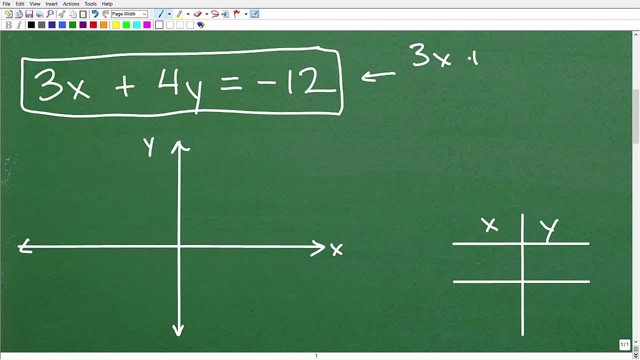 OK. so here we have three X plus four Y equals negative twelve. We have a nice whole number, integer value from the X. Same thing. We have a nice whole number in front of the Y, And then here we have a nice integer value over here. 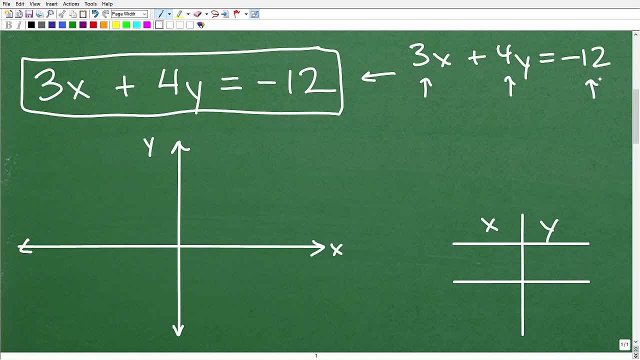 When a line is in this type of form, you always want to be thinking using the X- Y intercepts. We call this standard form. This line is in standard form or a X plus B. Y equals C. OK, so this line fits this format. versus the Y equals M X plus B form. 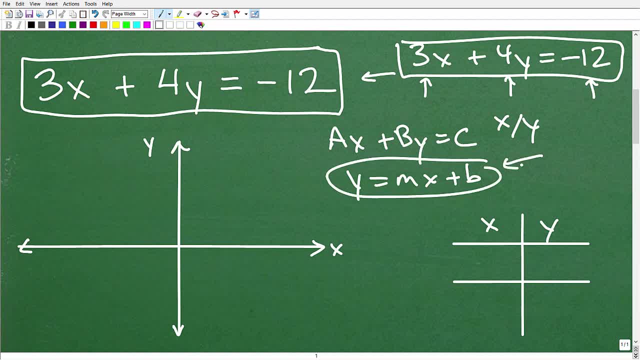 So if you see lines that are written in Y equals M, X plus B form, you want to graph them using that technique. If you see lines that are clearly written in the standard form, that particular format, you want to go ahead and use the technique I'm going to show you here now. 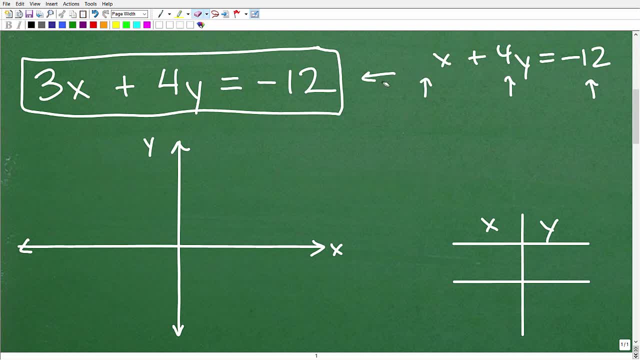 OK. so a big part of graphing Linear equations is just to first identify what form you know, is the line in. Now there are times where a line isn't in 100 percent, It's not clear, It's not in a particular format. 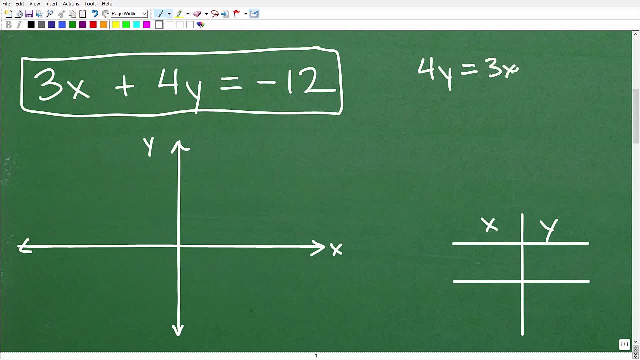 So in other words, if I had four Y equals three, X minus eight, well, that's not either in standard form or Y equals M, X plus B form. So you know, we have a choice there. We can either write it as Y equals or we can kind of put it into standard. 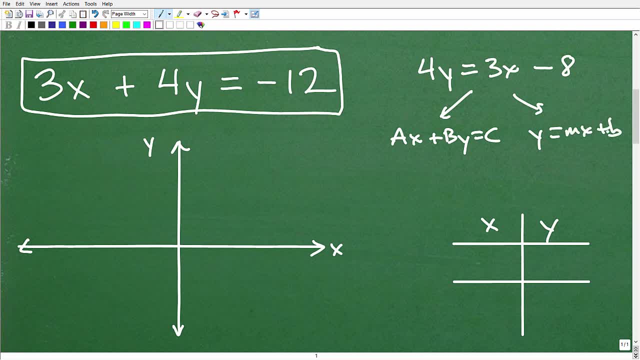 OK, Y equals M, X plus B, et cetera. OK, so you know again. the point of this video is to kind of clarify, really give you a good overarching understanding of linear equations and how to identify what form they're in and what your options are. 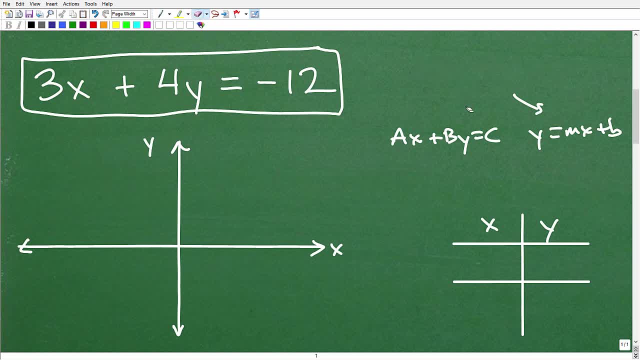 So you're going to need to know all these skills, But this particular problem is in a nice easy standard form setup. So, Knowing that we want to use X- Y intercept approach to we want to get the X and Y intercepts for this line. 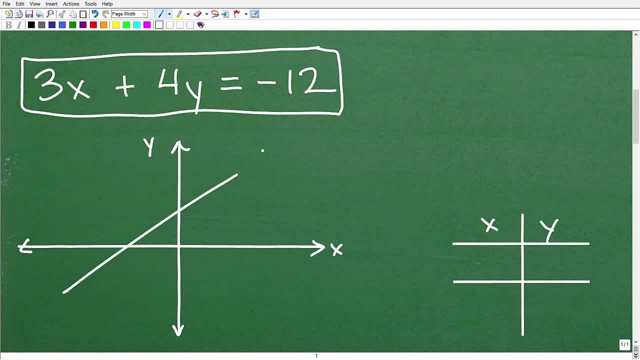 So I'm just going to just draw some sort of line like so here. OK, so just to identify what the X intercept and Y intercept is what. Well, how many points does it take to graph any line? Well, if I have a point here and another point here, I can draw the line. 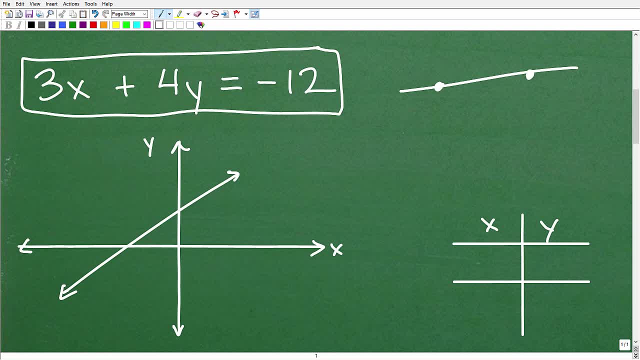 Right. So I need two points at a minimum. So what we're going to be going for is the X intercept And the Y intercept. So these are just the points where the line chops through the X axis. So, like right here, that would be the X intercept. 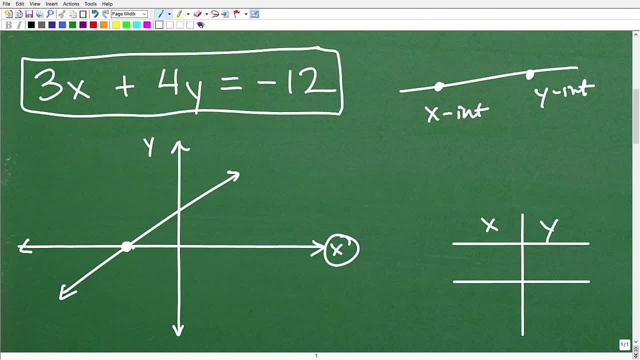 So this particular point is the X intercept. That's where it chops through the X axis And the line is chopping through the Y axis right there. So if I get this point and that point, I can, I can graph the line. So this is the whole idea behind the X- Y intercept. 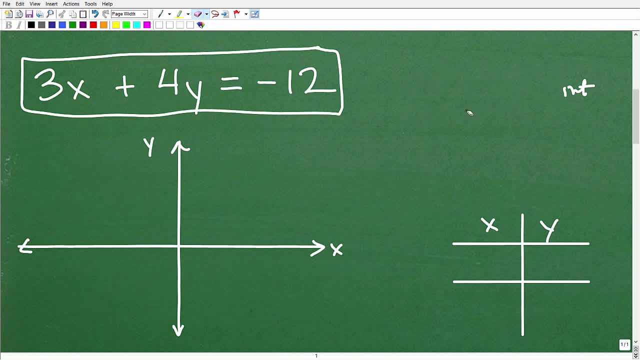 So that's where we're going to be going for in this Problem. OK, so how do we do that? Well, we're going to use a table of values, So here's how it works. All right, I'm going to put a zero here. X and Y. 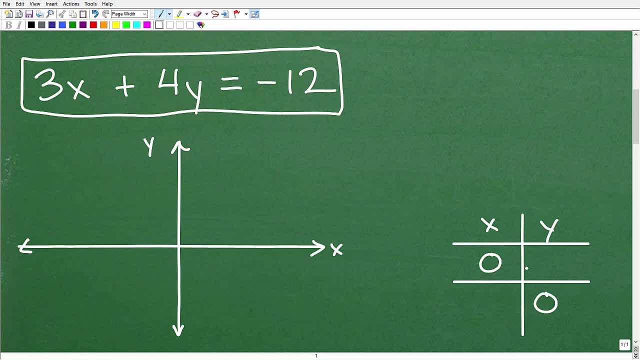 I'm going to put a zero for X and a zero for Y, And then I'm going to get these points This. you'll see how this works here shortly. OK, let's go ahead and figure out this table. We're obviously going to have to get this information right there for Y. 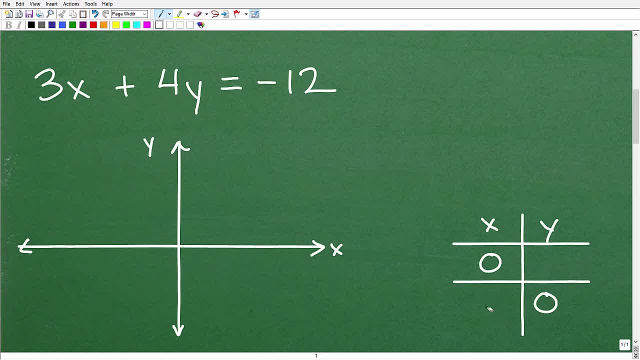 We're going to have to get this information right here for X. So here's what we do. So when X is zero, when X is zero- you look here I have the X column- when it's zero, What is Y? OK, well, let's go ahead and figure that out. 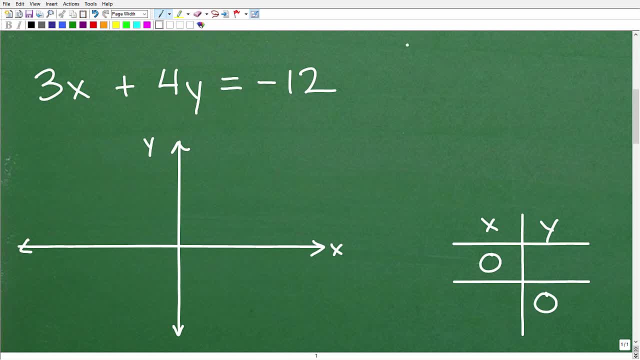 So we go over here to our our equation. All right, So three X plus four Y equals negative twelve And we're going to plug in zero for X. OK, that's what this is saying: Plug in zero for X, And I do that. 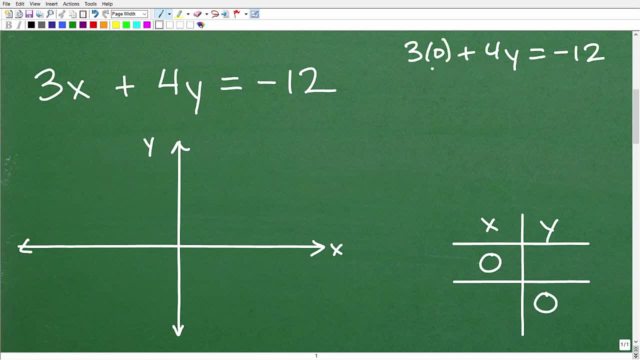 What I want to do now is solve this basic remaining equation for Y. So zero times Three is obviously zero. So I really need to solve this equation, for Y equals negative twelve, And hopefully all of you out there know how to do that. 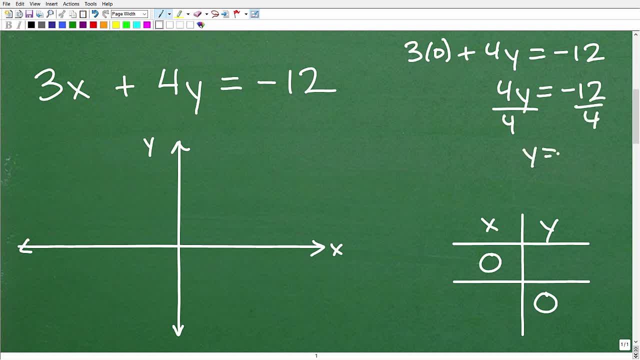 Just simply divide both sides of the equation by four And I get Y equals negative three. So that's what I would put right there: Zero negative three. OK, now, what's important about this? Well, let me just stop myself. 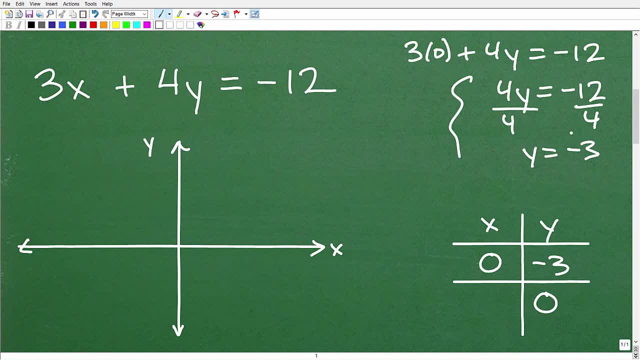 So if you were confused on how to do this, then you have to go back and do some additional review in algebra, Basic equation solving, et cetera. So remember algebra is all interlinked. OK, if you were like: oh, I understand this, but I always struggle with this part, 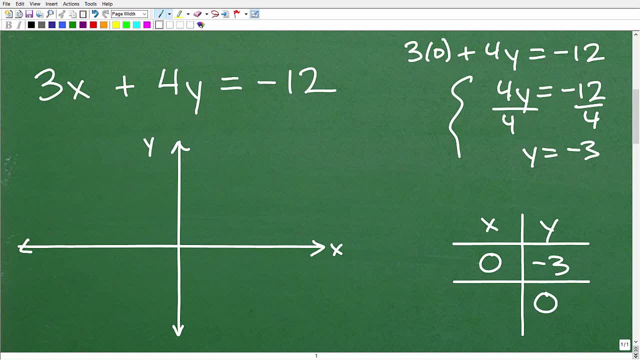 Well, that means you need to kind of, you know, review how to solve basic equations. OK, All right, So, so we plugged in zero, We got Y was equal to negative three. But what is the importance of that? OK, well, this, this right here is a coordinate. 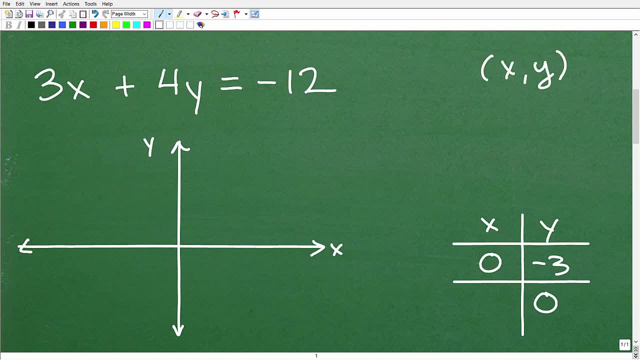 It's an X, Y point, All right, And it's at zero, negative three. So zero, negative three is on this line, OK, so let's go and plot that point real quick: Zero, X is zero and Y is negative three. Let's say that: one, two, three. 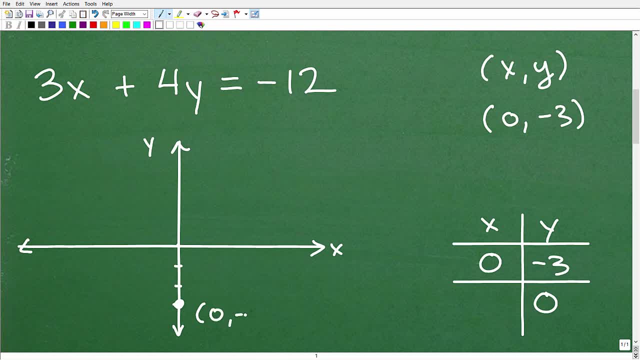 Let's call it right there. OK, that's zero negative three. Here's the point. And what would that point be? Is that my X intercept or Y intercept? All right, so that's the Y intercept, because that's the point. this line is going to chop through on the Y axis. 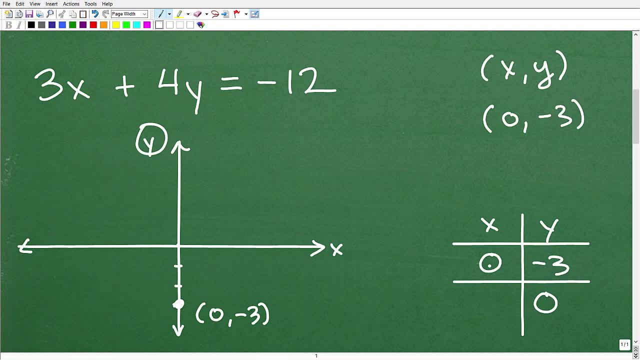 OK, so we get the Y. We get the Y intercept when X is zero. OK, now we're going to get the X intercept. We're going to do the same thing, But this time we're going to plug in zero for Y and and solve for X. 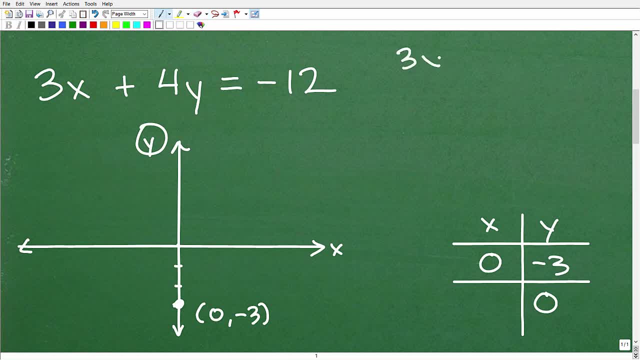 OK, so let's go and do that now. So three X plus four Y equals negative twelve. So this time we're going to plug in the zero for Y. OK, we'll erase that and we're going to solve for X. So four times zero, of course, is zero. 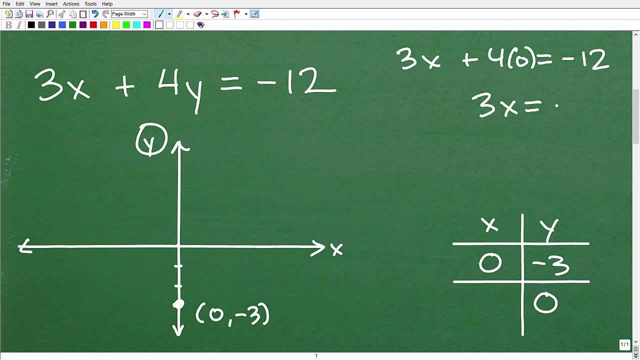 So we're going to solve This problem right here. three X equals negative twelve, And when I divide both sides of the equation by three, I get X equals negative four. OK, X equals negative four. So that is going to be the corresponding coordinate, of course, is going to be negative four, zero. 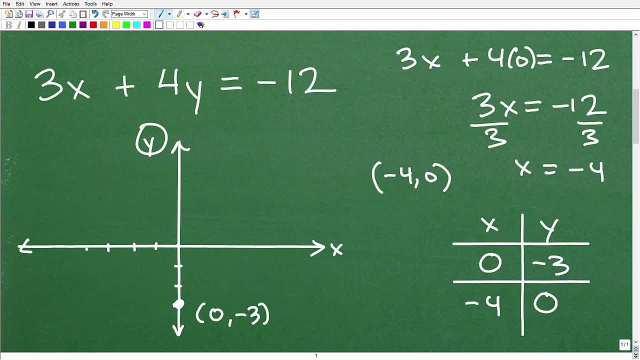 So it's going to plot that that's going to be one, two, three, four negative four right there on the X axis. OK, there's negative four, Zero, OK. so now I have a point here. That's my X intercept. 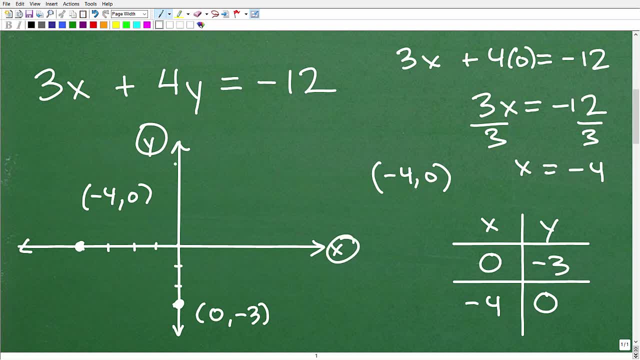 All right, because this is the X axis and this is my Y intercept. So now I just draw a line. We kind of carefully do that, And there you go Right. So I drew a line through those two points. Again, this is my Y intercept and this is my X intercept. 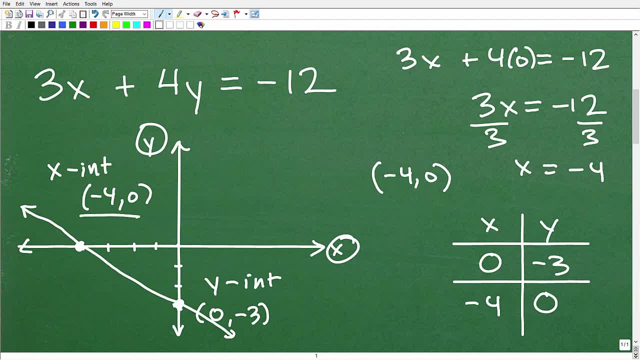 All right, X intercept is located here, Y intercept is located here, So you just can't go wrong with using the table to find out what the X and Y intercepts are. This is really standard stuff And it's going to be a real basic question that you're going. 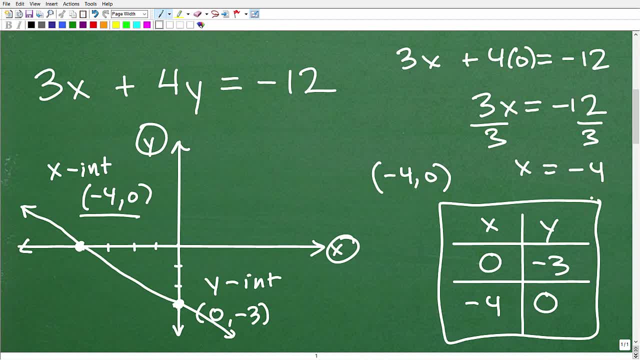 to to face you know in your class- for sure It's your teacher- and say: hey, you know, tell me what the X and Y intercepts are. You need to go ahead and know how to calculate that Now. this also works. 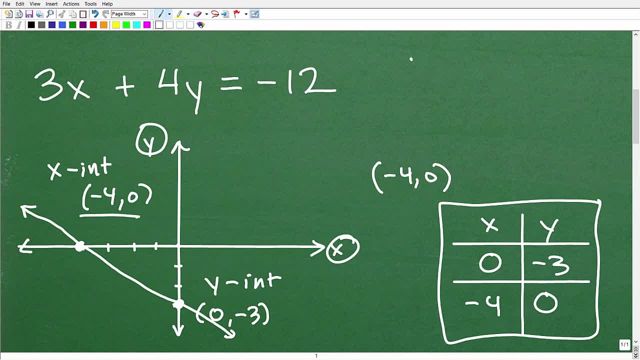 OK, this concept, what I just told you about. even if you had a line written in this form: Y equals three, X plus seven, You could still use this table of value, just like that, to locate the X and Y intercept. So again, you know it takes two points on the X- Y plane to plot a line.